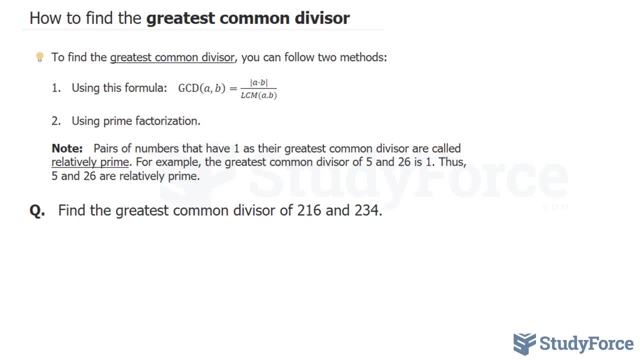 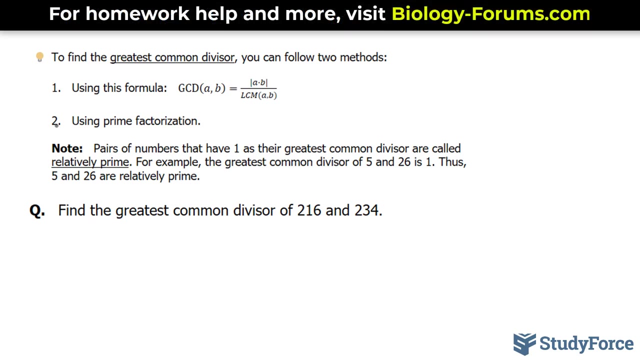 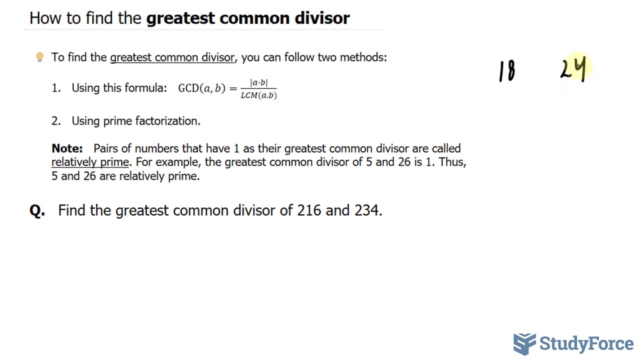 In this lesson, I'll show you how to find the greatest common divisor. To find the greatest common divisor, you can follow two methods. You can use this formula, or you can use prime factorization, and we've dedicated one video to that. already Now, just to give you an idea of what this means, let's say we have the number 18 and the number 24.. Both of these numbers are divisible by 2, although that's not the greatest common divisor, The greatest common divisor is the number 18.. 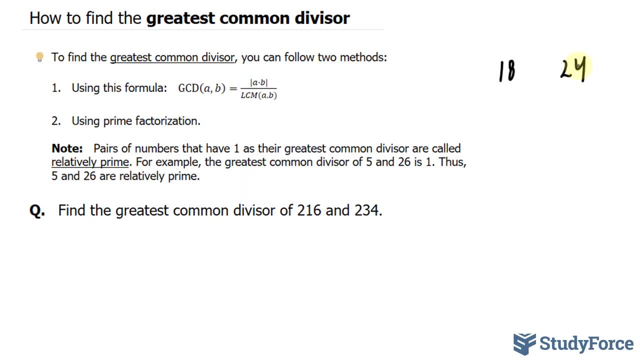 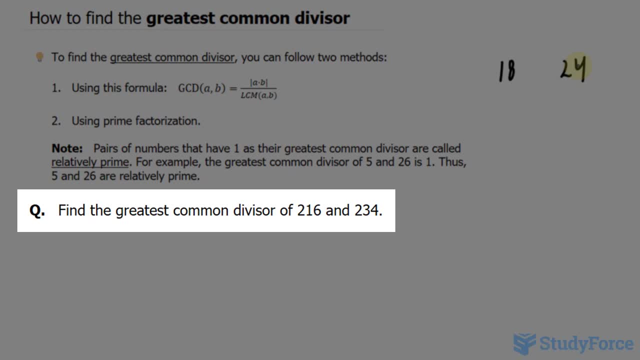 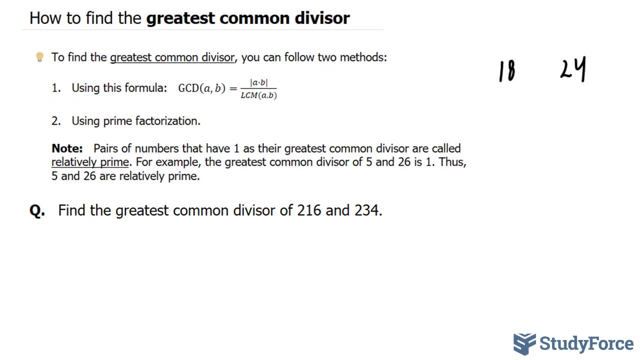 The greatest common divisor here would have to be 6.. So I'm going to show you a method on how you can find that. The question reads: find the greatest common divisor of 216 and 234.. First I'll show you this method where we use the formula, and the formula is easy to follow. What we do is we start by multiplying the two numbers A and B at the top, And if the two numbers are negative, remember we're taking the absolute, which means that in the end your answer has to be positive. So we'll take 216 and 234.. 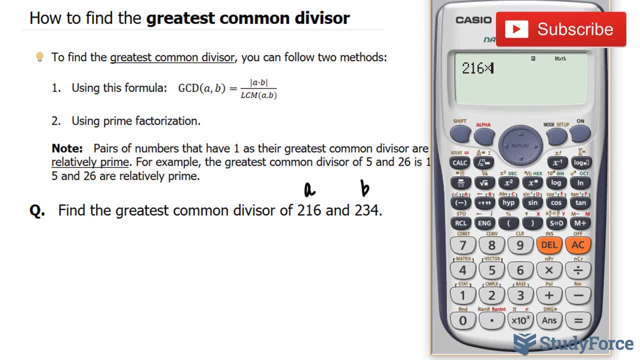 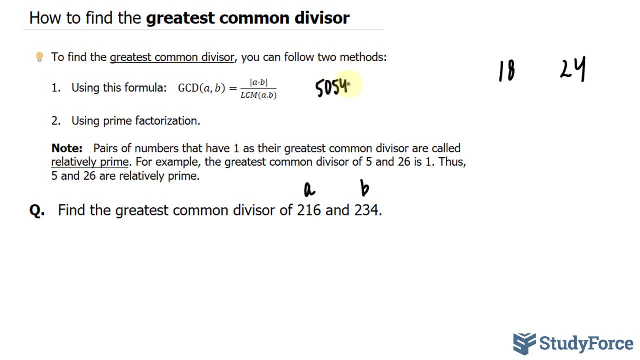 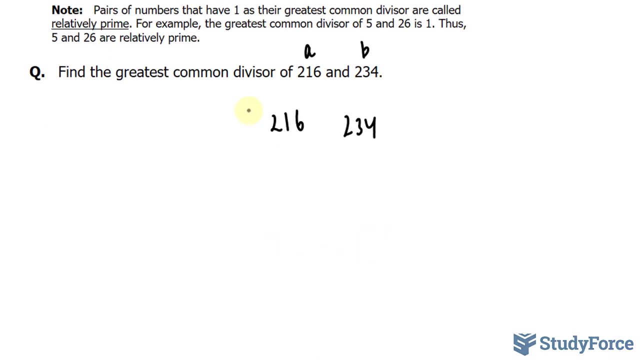 So we'll take 216 and multiply it to 234.. 216 times 234. We end up with 50,544.. So that's the top part, 5544 divided by the lowest common multiple. To find the lowest common multiple of 216 and 234, we'll write down 216 and 234. And we'll divide this by its prime factors. A prime factor that divides into both of these equally is 2.. 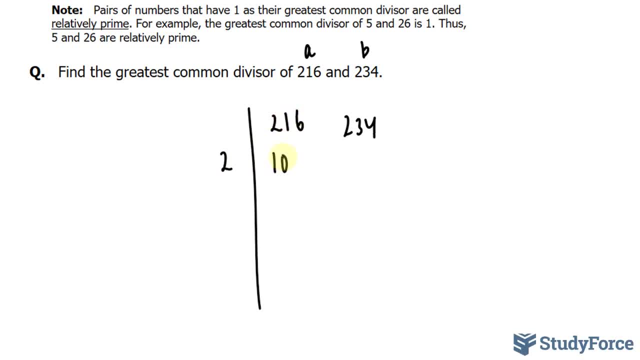 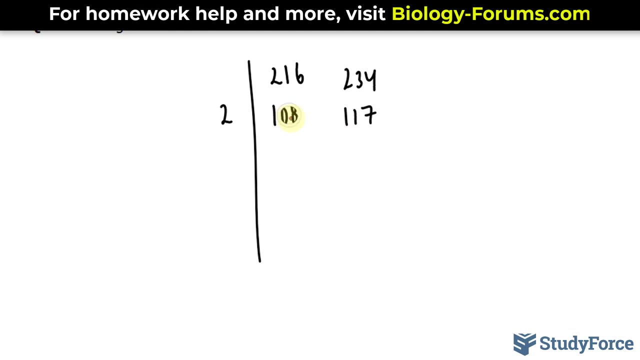 216 divided by 2 is 108.. And over here is 117.. Next, let's find a number that divides into these two, if we can. This is divisible by 3, and so is this, because 1 plus 0 plus 8 is equal to 9.. 9 is divisible by 3, so is this. 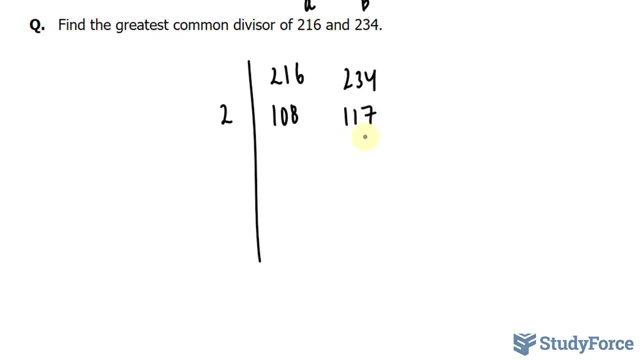 In the same case here: 1 plus 1 plus 7 is 9.. That's divisible by 3.. So I'm going to write down 3.. 108 divided by 3 is equal to 36.. So I'm going to write down: 3.. 108 divided by 3 is equal to 36.. 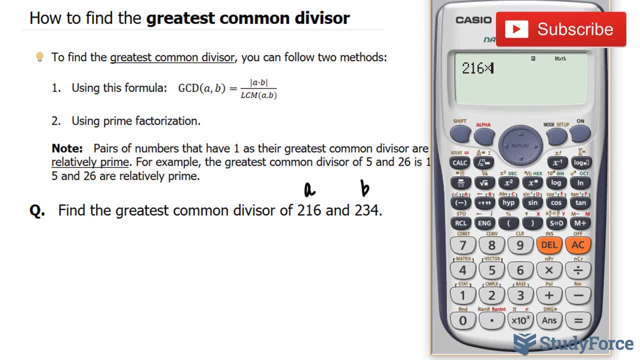 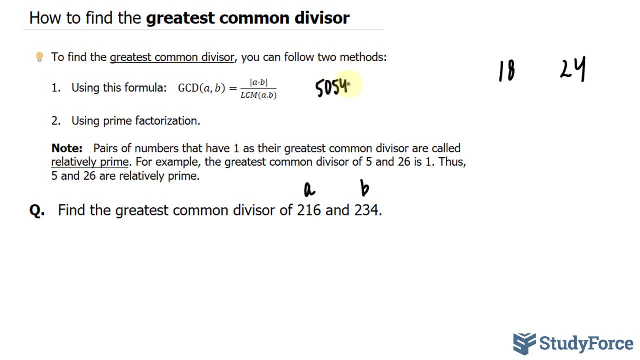 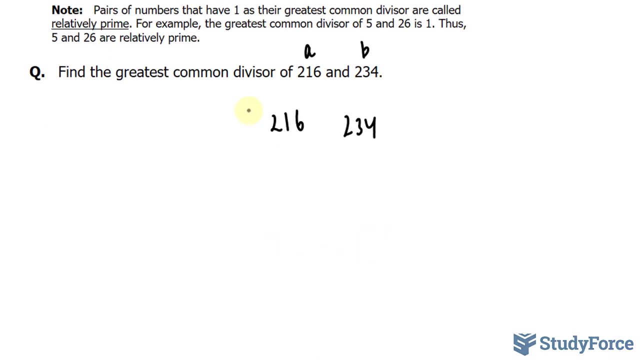 216 and multiply it to 234.. 216 times 234. We end up with 50,544.. So that's the top part, 5544 divided by the lowest common multiple. To find the lowest common multiple of 216 and 234, we'll write down 216 and 234. And we'll divide this by its prime factors. A prime factor that divides into both of these equally is 2.. 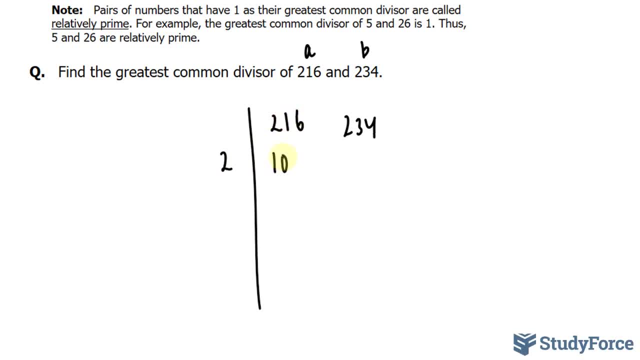 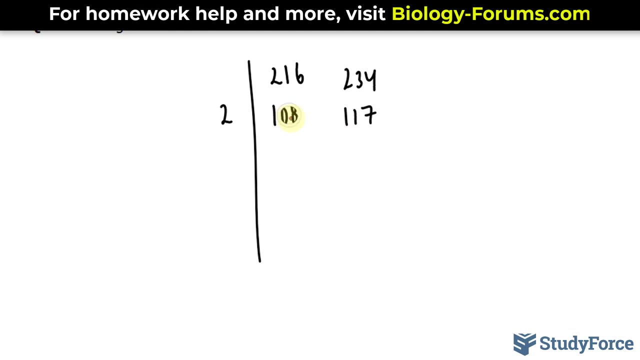 216 divided by 2 is 108.. And over here is 117.. Next, let's find a number that divides into these two, if we can. This is divisible by 3, and so is this, because 1 plus 0 plus 8 is equal to 9.. 9 is divisible by 3, so is this. 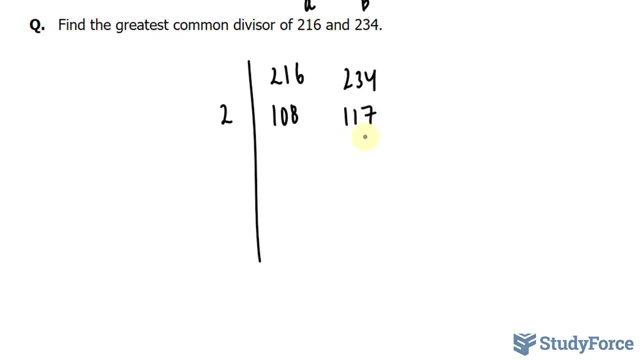 And the same case here: 1 plus 1 plus 7 is 9.. That's divisible by 3.. So I'm going to write down 3.. 108 divided by 3 is equal to 36.. So I'm going to write down 3.. 108 divided by 3 is equal to 36.. 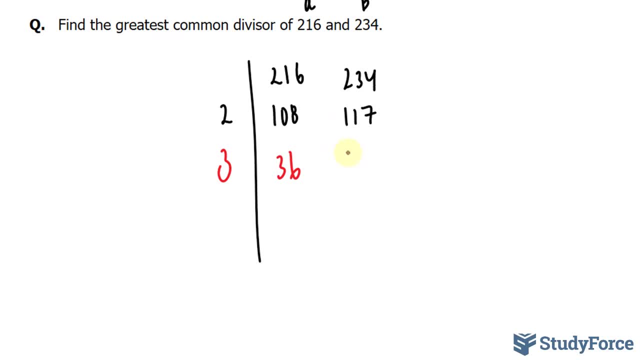 And 117 divided by 3 is equal to 39. Now this is also divisible by 3.. Both of them are, So I'll write down another 3.. This becomes 12. And this becomes 13.. Next, I'll divide this number by 2.. This becomes a 6. And I'll keep this as 13 because it's not divisible. 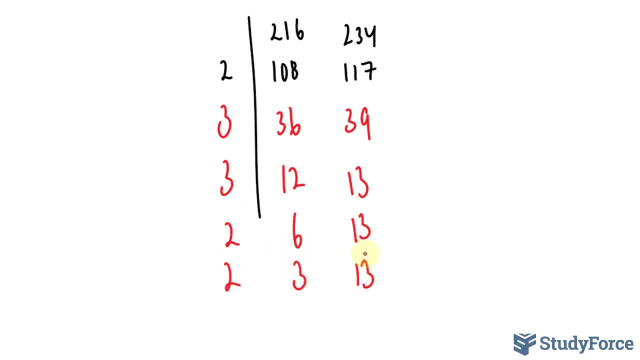 Again by 2, that becomes a 3.. That's a 13.. Divide this by 3.. That becomes a 1.. I don't have to worry about that anymore. Divide this by 3.. That becomes a 1.. I don't have to worry about that anymore. 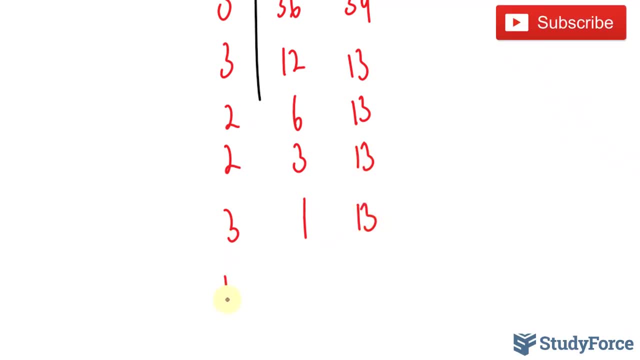 And we're left with 13.. That's a prime number, So I'll write down 13. at the end, I'll multiply 2, 3, 3,, 2,, 2, 3, and 13.. Whatever we end up with our product, we'll divide by 5544, which we found earlier. 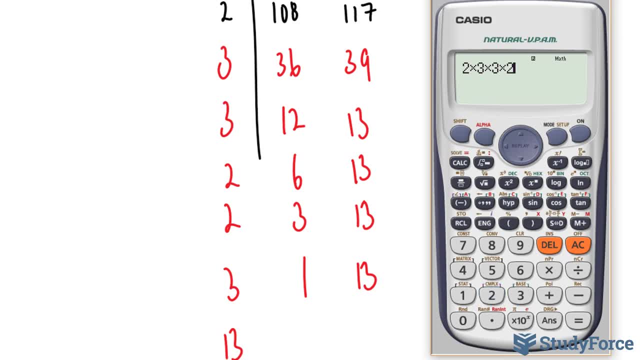 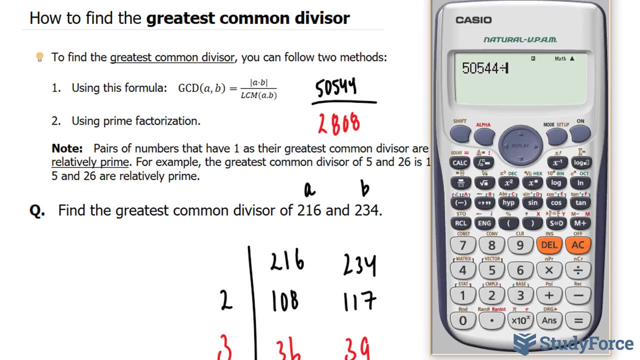 2 times 3 times 3 times 2 times 2 times 3 times 13.. And we end up with 2808.. So I'll write that here: 2808 using my calculator, 5544 divided by 2808.. And we end up with 18.. 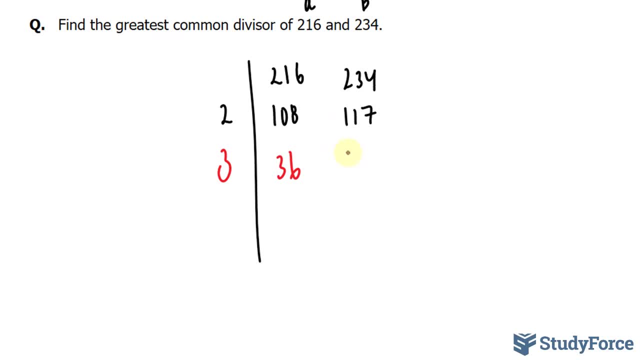 And 117 divided by 3 is equal to 39. Now this is also divisible by 3.. Both of them are, So I'll write down another 3.. This becomes 12. And this becomes 13.. Next, I'll divide this number by 2.. This becomes a 6. And I'll keep this as 13 because it's not divisible. 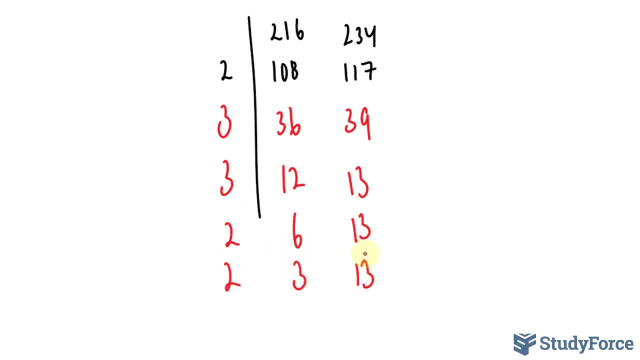 Again by 2, that becomes a 3.. That's a 13.. Divide this by 3.. That becomes a 1.. I don't have to worry about that anymore. Divide this by 3.. That becomes a 1.. I don't have to worry about that anymore. 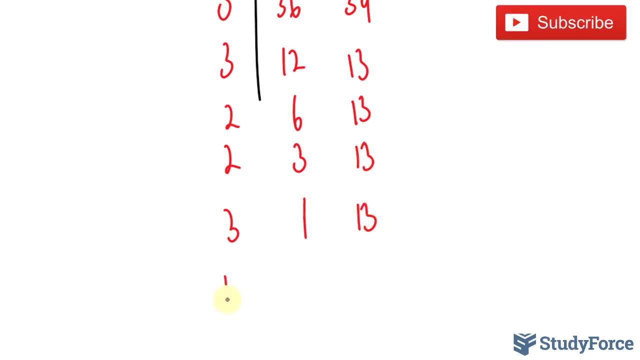 Divide this by 3.. That becomes a 1.. I don't have to worry about that anymore, And we're left with 13.. That's a prime number, So I'll write down 13 at the end. I'll multiply 2,, 3,, 3,, 2,, 2, 3, and 13.. 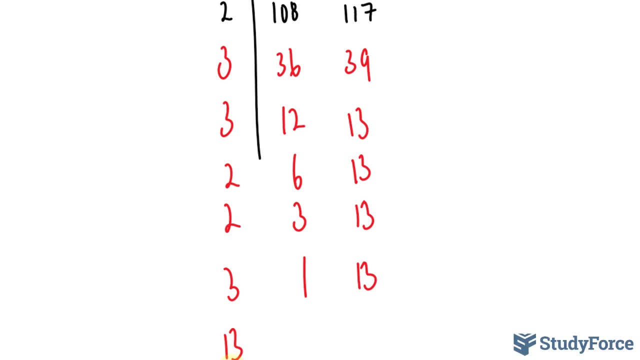 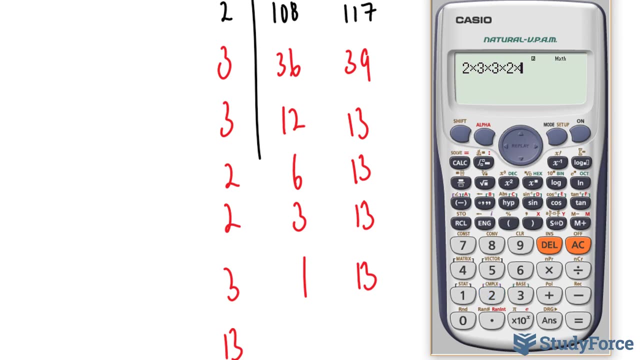 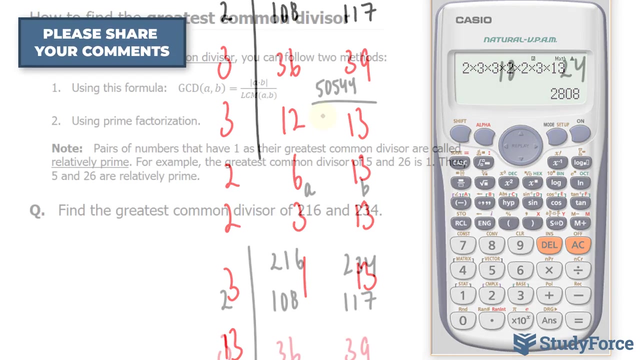 Whatever we end up with our product, we'll divide by 5544, which we found earlier- 2 times 3 times 3 times 2 times 2 times 3 times 13.. And we end up with 2808.. So I'll write that here. 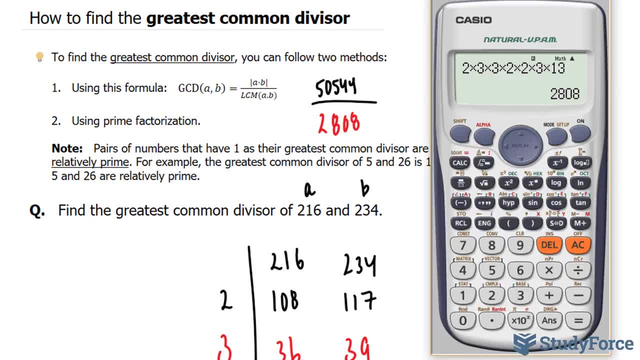 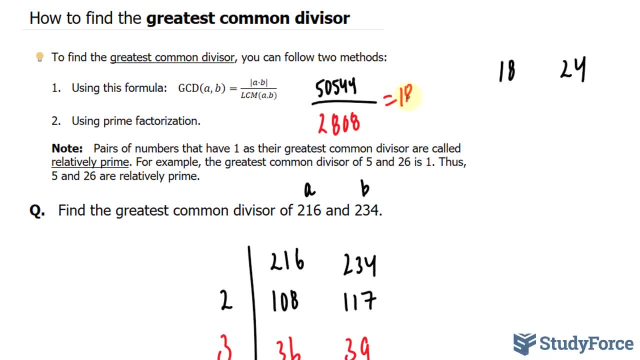 2808.. Using my calculator, 5544 divided by 2808.. And we end up with 18.. And you can test if this is correct by dividing both of these by 18. And you will find out that they're divisible. 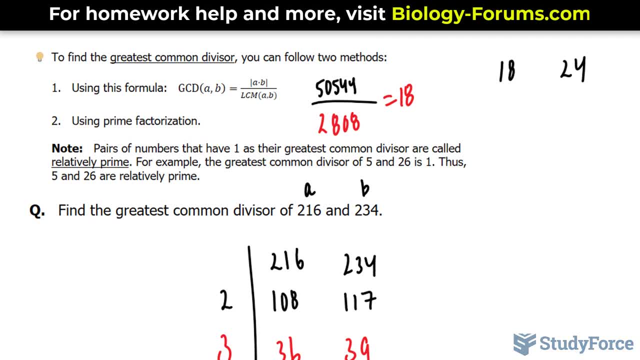 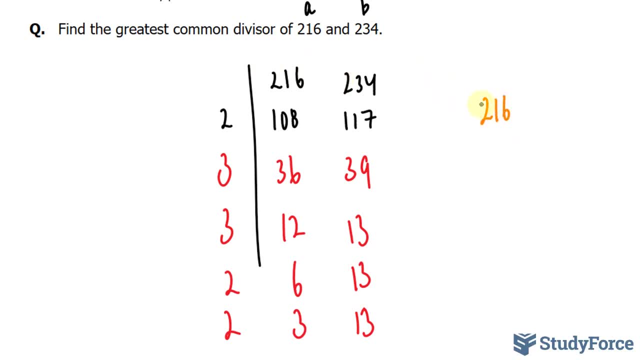 There's a second method and you can use the prime factorization method. We have a video dedicated to prime factorization, So we'll create a tree for both numbers. I'll write down 216 and divide this by prime numbers. I'll start with 2.. 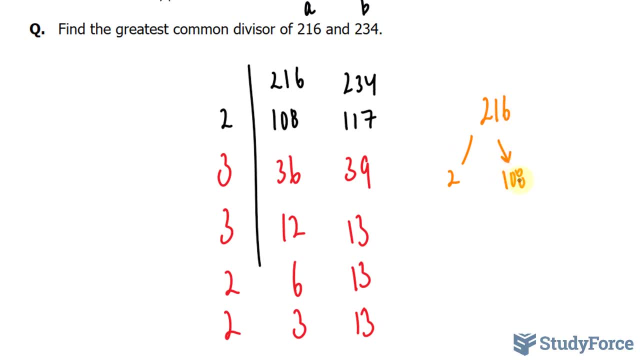 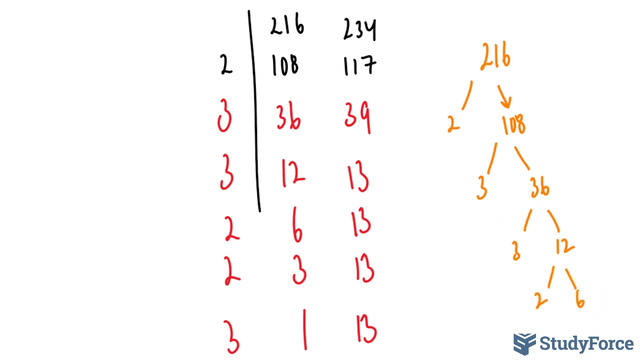 216 divided by 2 is 108.. Now I need to divide 108.. We found out that this is divisible by 3, so I'll do that. This becomes 36.. 36 is divisible by 3, again 12,, 2, 6,, again 2, 3, and we found our prime factors. 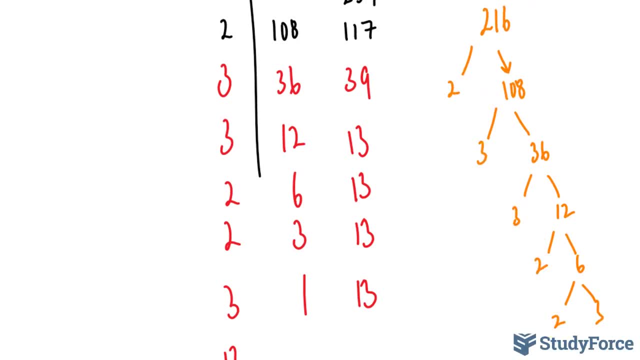 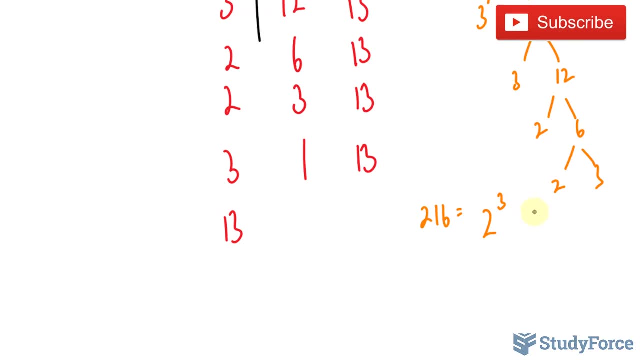 2, 3,, 3,, 2,, 2, and 3.. So I'll write down: 216 is equal to 2 to the power of 3, and 3 to the power of 3.. Because we had two 3s. 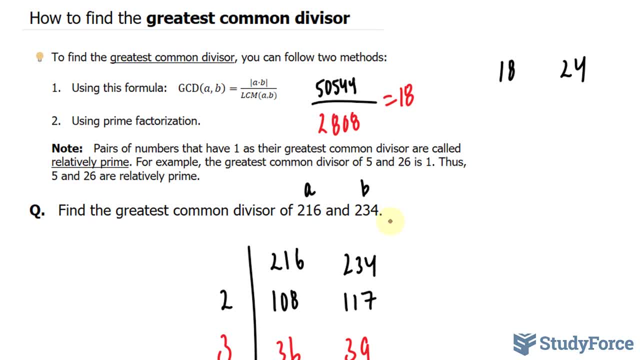 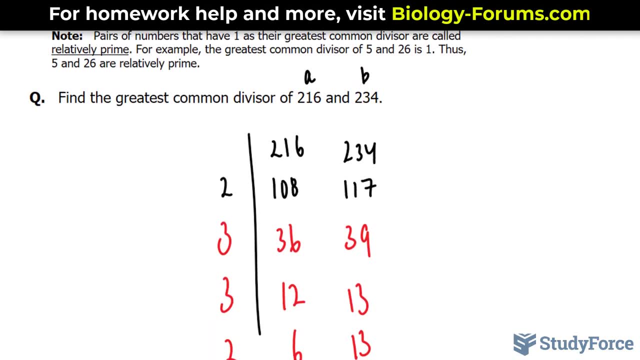 And you can test if this is correct by dividing both of these by 18.. And you will find out that they're divisible. There's a second method and you can use the prime factorization method. We have a video dedicated to prime factorization. 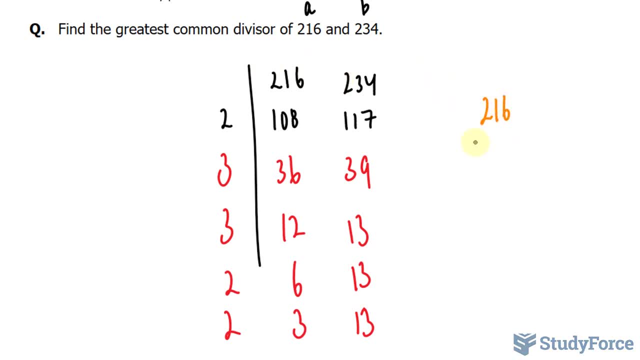 So we'll create a tree for both numbers. I'll write down 216 and divide this by prime numbers. I'll start with 2.. 216 divided by 2 is 108.. Now I need to divide 108.. We found out that this is divisible by 3, so I'll do that. 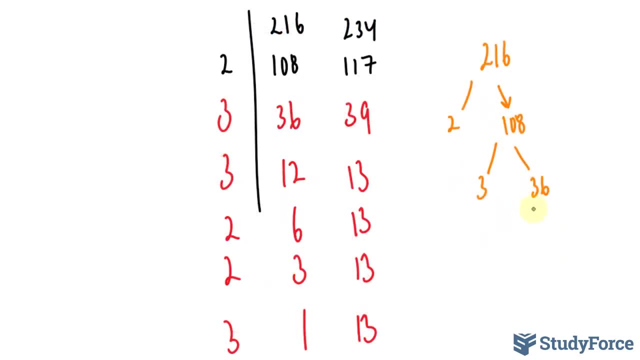 This becomes 36.. 36 is divisible by 3, again 12,, 2,, 6,, again 2,, 3, and we found our prime factors: 2,, 3,, 3,, 2,, 2, and 3.. 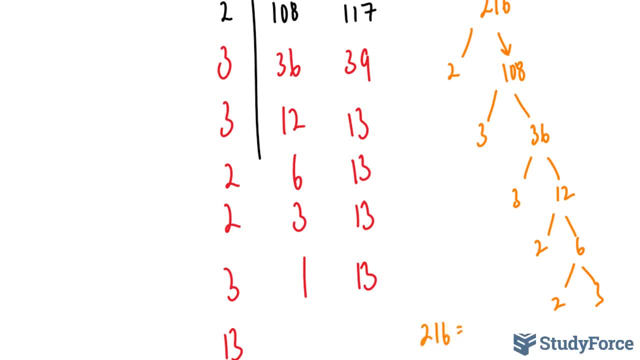 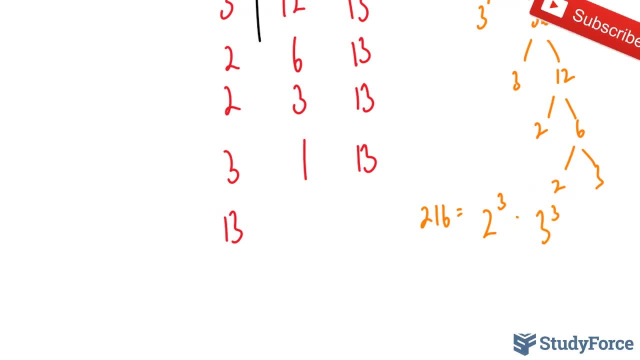 So I'll write down: 216 is equal to 2 to the 3rd, So we'll divide the power of 3 and 3 to the power of 3. Because we had two 3's: 1,, 2, and 3.. 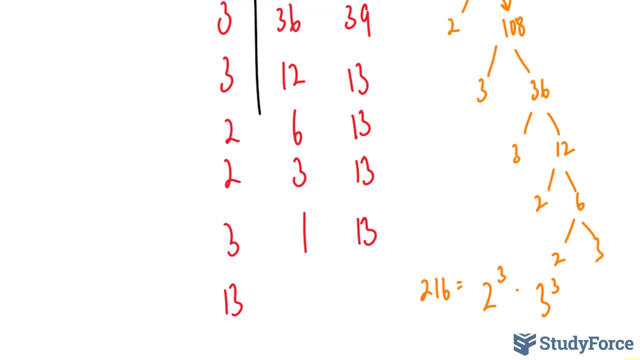 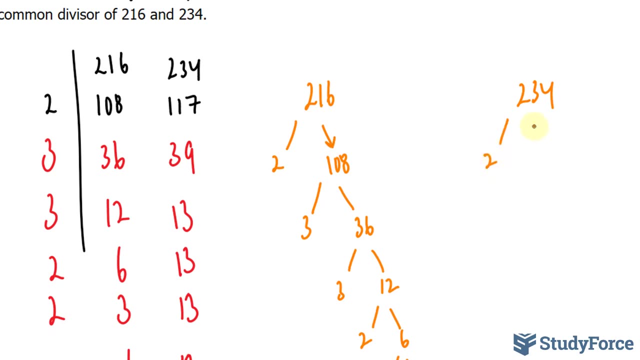 And we had three 3's as well. So we'll do the same thing for the other number. We'll create a tree: 234.. We'll divide this by 2. 117.. Divide this by 3. 39.. 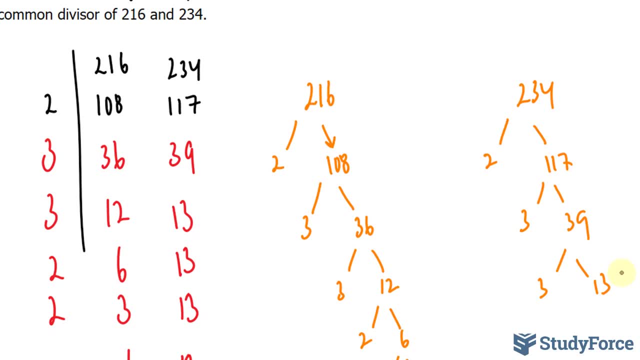 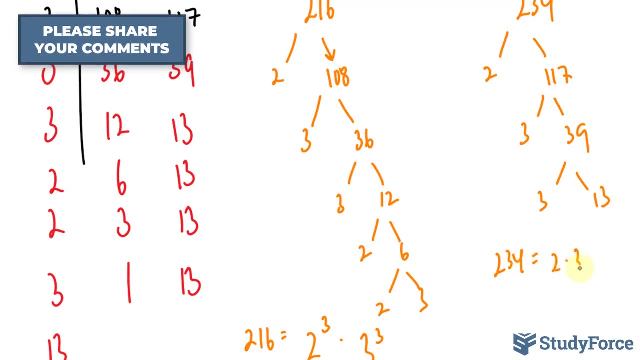 3,, 13.. And that's it: 2,, 3,, 3, and 13.. 234 is equal to 2 times 3, to the power of 2 times 13.. Now, at this stage, once you find the prime factorizations of both numbers, 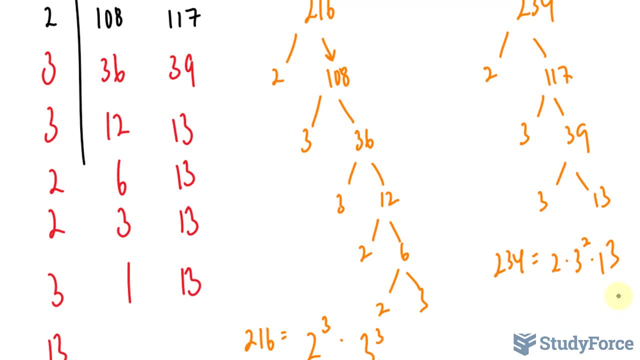 we have to select each prime factor with the smallest exponent that is common to each of the prime factorizations. So which exponent is appropriate for 2 and 3?? We choose the smallest exponent. So out of these two, these two 2's, we'll choose this one. 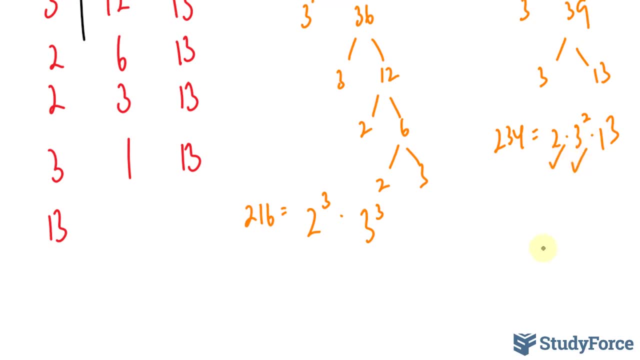 And we'll divide this by 2.. I'll choose 2.. I'll choose this. 3. And 13 is not common, So we're not going to include that. We'll take 2 times 3 to the power of 2.. 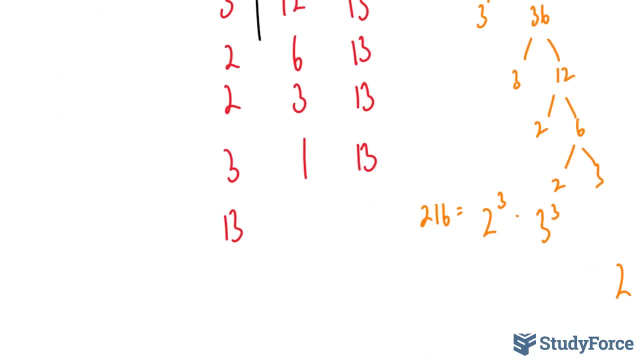 And that is equal to 18.. And there you have it: Two methods on how to find the greatest common divisor.